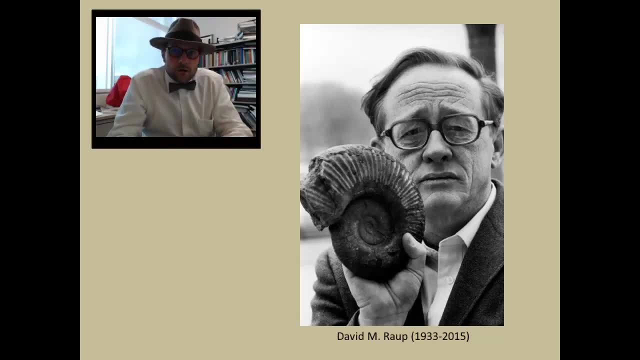 David Raup was an unusual paleontologist at the University of Chicago who worked principally in front of a computer and rarely in the field. His interest was in quantifying the quality and nature of the fossil record from published works. His interest was in studying the patterns of extinction and the diversity of life. 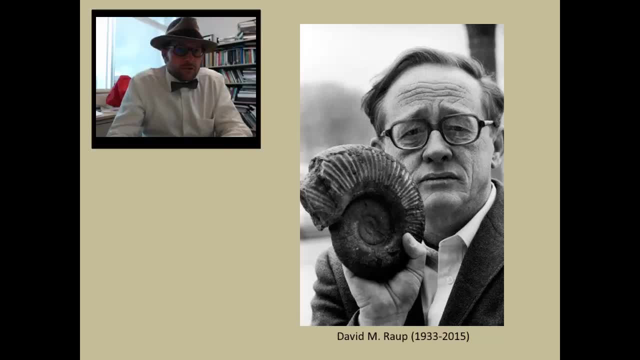 We'll read more about Raup and his work throughout this semester. In this lecture, I am going to simplify some of Raup's work as well as discuss how a basic examination of what we know in the scientific literature can help us address the question. 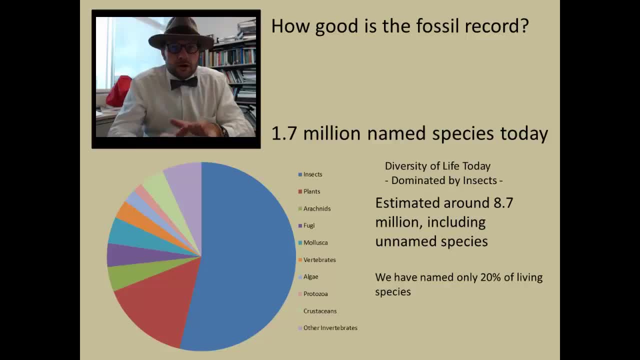 how good is the fossil record? The first number we need to uncover is how many species are living today. This is not an easy number to find. If we simply add all the unique names of species, We find that there is About 1.7 million species which have names assigned to them. 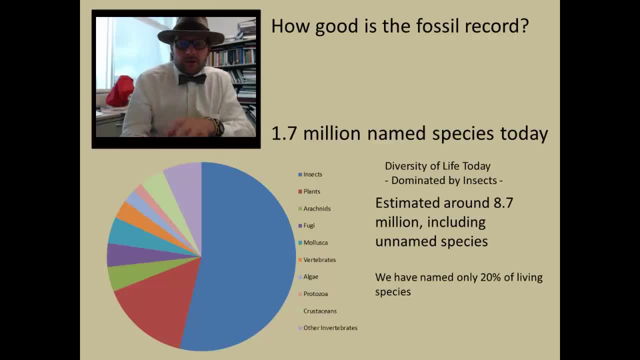 If you were to do a Google search, you would find a much higher estimate of 8.7 million species, which is just an estimate. In fact, scientists really don't know how many living species there are. We just keep discovering new ones every year. 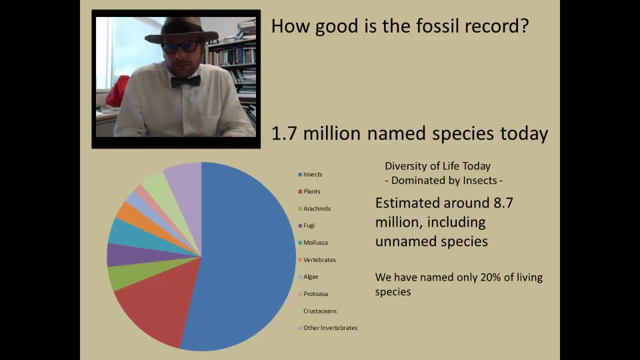 In fact, if the 8.7 million species 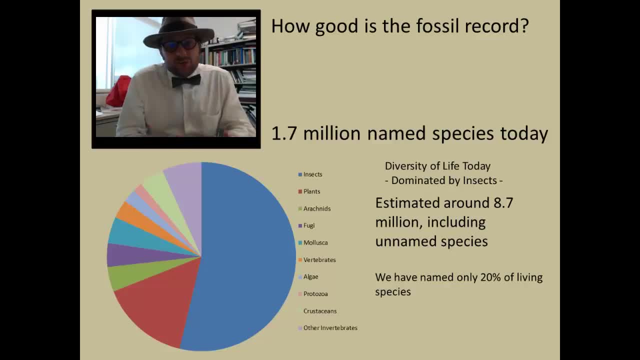 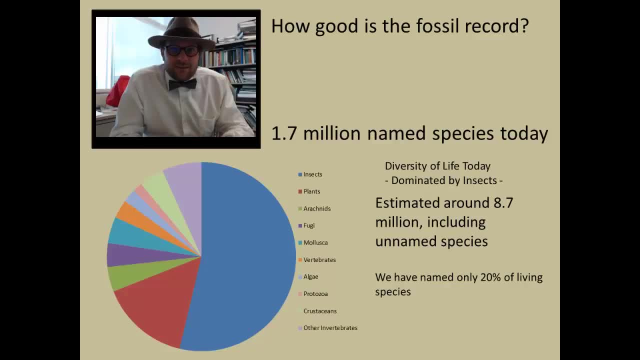 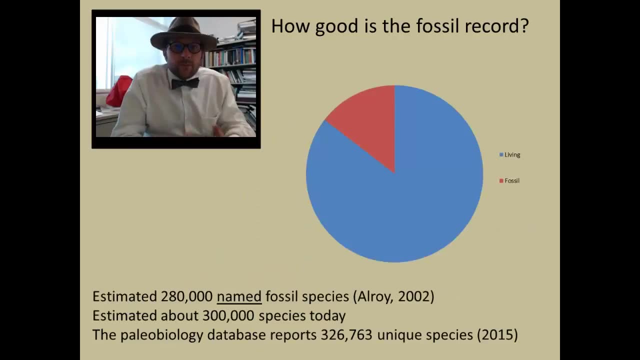 Now that we have a vague idea of the number of living species, how about the number of fossil species only known from the fossil record? Well, that number is rather small compared to the 1.7 million named species. John Alroy was the last to publish a good survey in 2002, and found about 280,000 named. 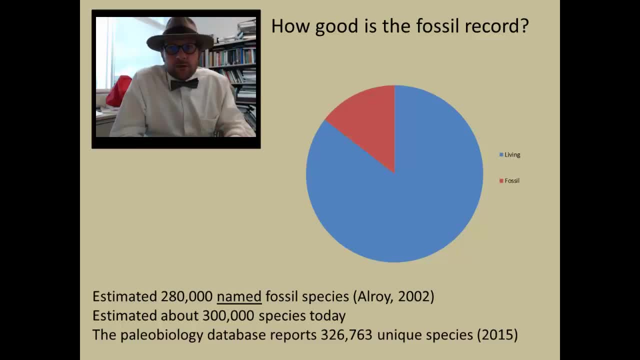 species known from the fossil record. More recent estimates are near 300,000 named species known only from the fossil record. The Paleobiology database reports about 326,000 living species with fossil records, so the 300,000 named species is a good estimate. 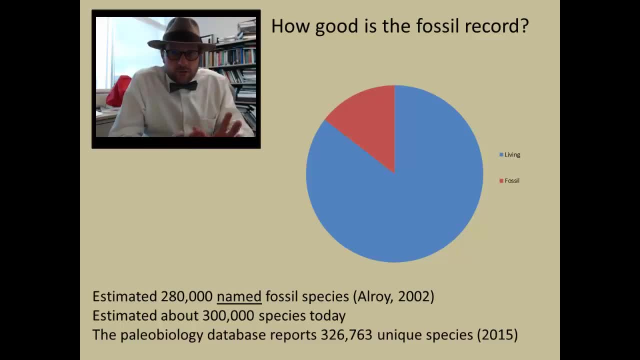 If we add these additional species into our pie chart of now 2 million living and fossil species, the vast majority of named species are living. This comparison gives us a hint at how few fossils are known of the 99.99% of life that 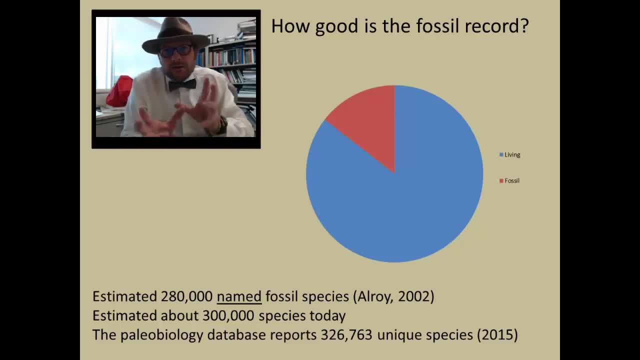 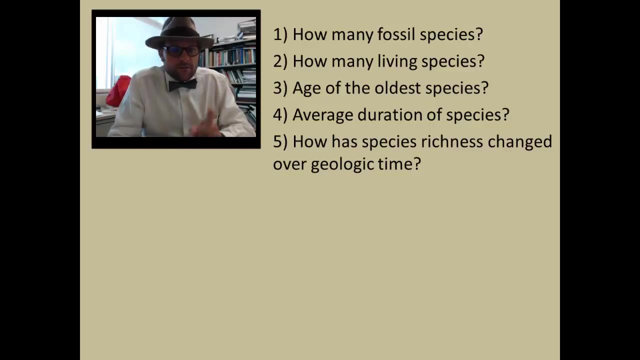 has gone extinct, But what we still want to know is how many species have ever existed, and compare this estimate to what we have discovered so far in the fossil record. To do this, we need to know a couple things: 1. How many fossil species are there? 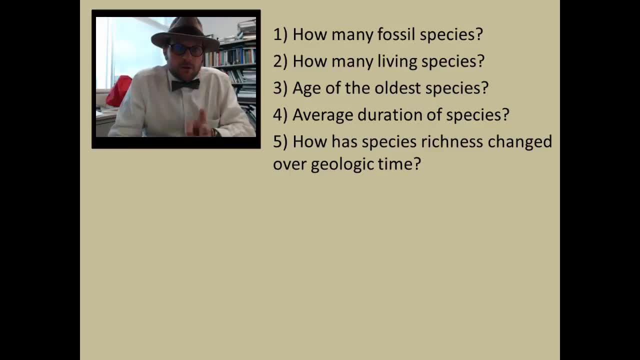 2. How many living species are there. 3. How many fossils are there. 3. The Age of the oldest species. 4. The average duration of the species. 5. How has species richness changed over geological time? 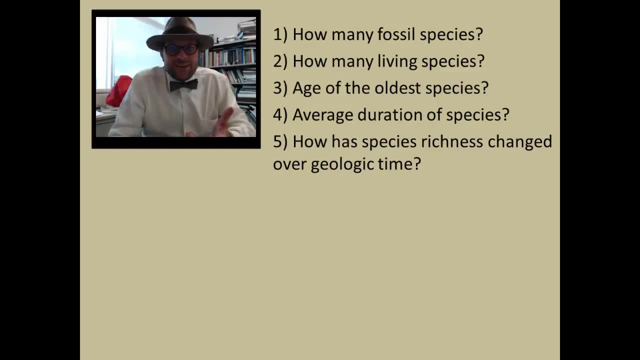 Each of these are really big questions in paleontology and in this lecture I will answer them extremely simplistically in order to start a discussion. The true answers to these questions are hotly contested in paleontology. For question 1. many fossil species are known. we will use the figure 300,000.. 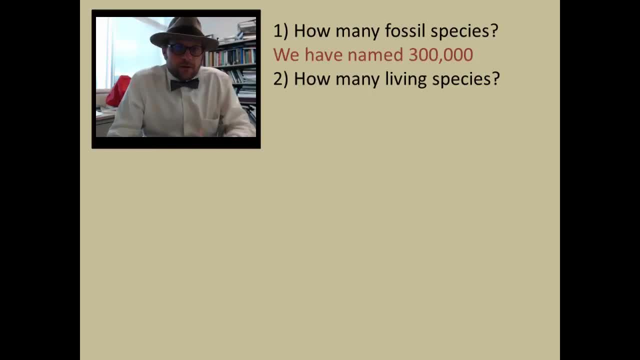 For question 2, how many living species? we will use the modest figure of 1.7 million species, noting that it is likely an underestimate of the true number, which could be as high as 8.7 million. For question 3, we will root our species at 600 million years ago. 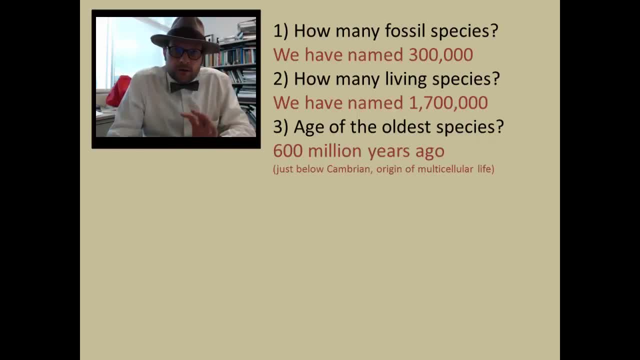 Clearly, life evolved much earlier than this date. Most states have this- around 3.8 billion years ago. However, we are mostly interested in multicellular life, and the number of species known prior to 600 million years is much lower than after 600 million years and 600 million years ago. 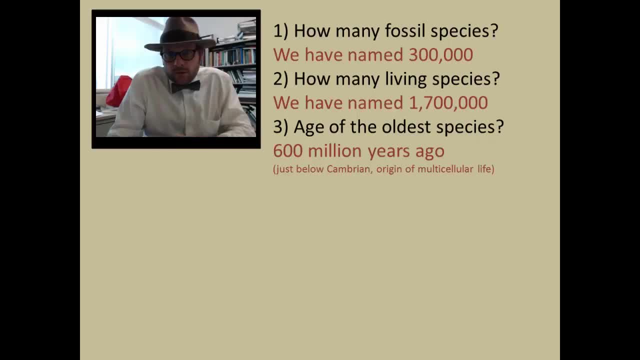 life was rapidly diversifying. We will talk more about early life during the Precambrian period later on this semester. For question 4, the average duration of species, there has been a lot of estimates for duration of species in the fossil record, which varies between groups. 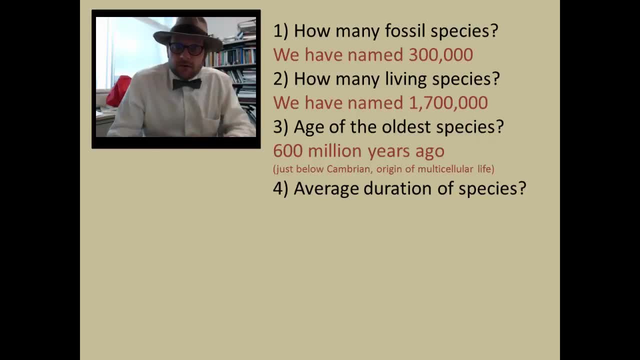 Some groups, like mollusks, have long durations in the fossil record, near 10 million years, while other groups, like mammals, have short durations, around 1 million years. For the sake of simplicity in this study we will use the figure of 4 million years. 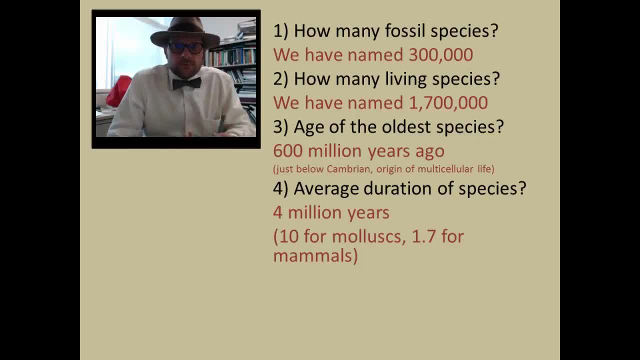 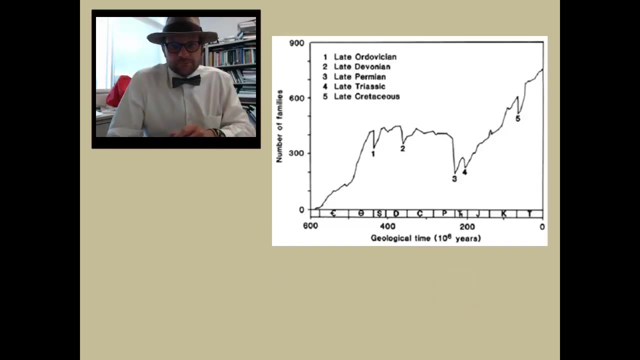 as the average duration for a species in the rock record. For question 5, how species richness has changed for geological time. we will need to look at a prediction. This figure is a chart of the number of fossil marine invertebrate families over geological 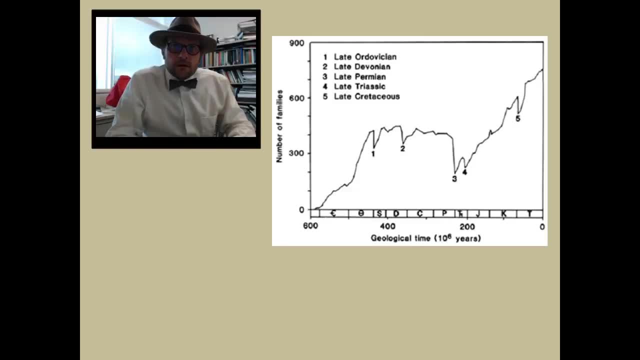 time, first developed by Jack Stabansky. The graph has been called the Stabansky curve. You can see five major extinction events, each numbered, but between each of these mass extinction events the number of taxa or groups has grown. 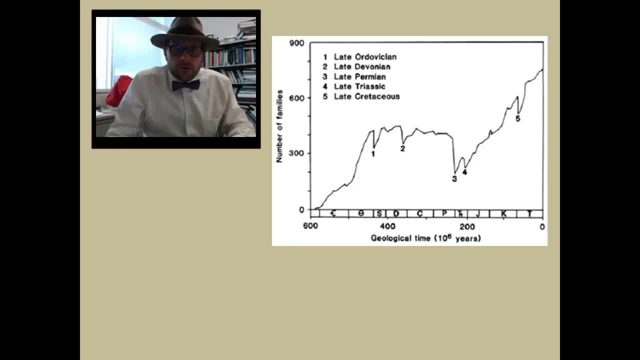 To keep things really simple, we will convert this curve into a triangle, which approximates the same dimensions of the original curve. Using this approximate triangle, we can get an estimate of the total number of species that have ever lived. by using the geometric formula for the dimensions of a triangle of species divided by the average species duration. Doing this, we get a big number: 127.5 million species existed. Using this number, which is likely a low estimate compared with the 300,000 known species, we can estimate the total number of species that have ever lived. 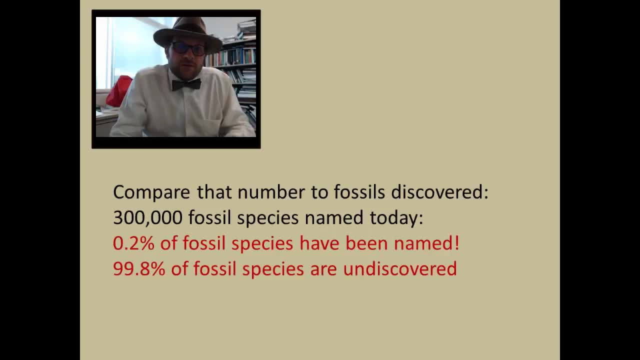 Using this number, we can estimate the total number of species that have ever lived. Using this and the figure from the rock record that we take, we can have 0.2% of extinct species known by scientists, of which 99.8% is unknown to scientists. 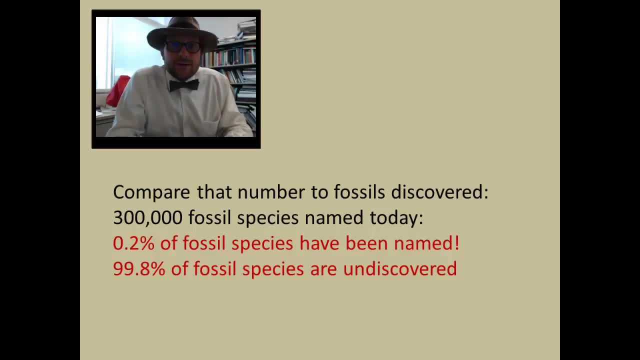 Using this along with the taco scale, we find that 29,000,000 species have ever lived. Owing to this variable, 99.99% of life is extinct is an acceptable estimate, however. 98.7% of life is extinct. 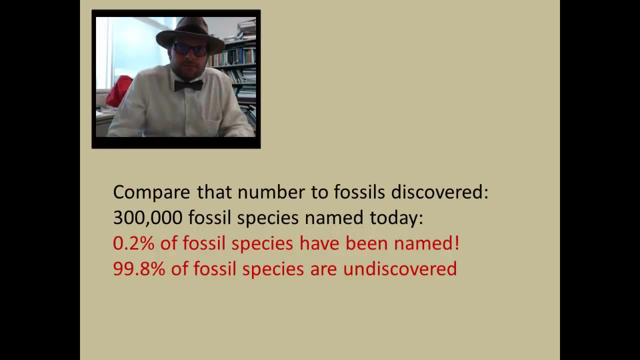 If we do the math chicken and take the uzcelllet fissure, the value is not going to get richer than the fissure that moves on an existing crop- an under estimate. This is really not very good, because what can we tell from 0.2% of the species preserved? 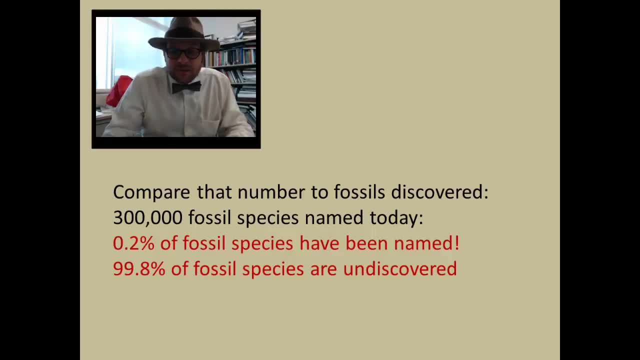 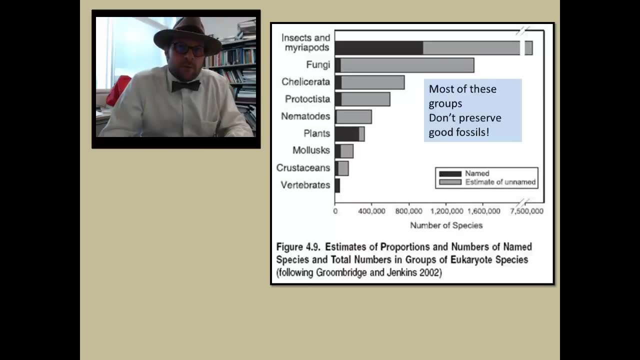 in the fossil record about the history of our planet. This may not be as bad as it seems If we look at the number of living species. most living species are members of groups that don't preserve great fossils, groups such as insects, fungi and nematodes. 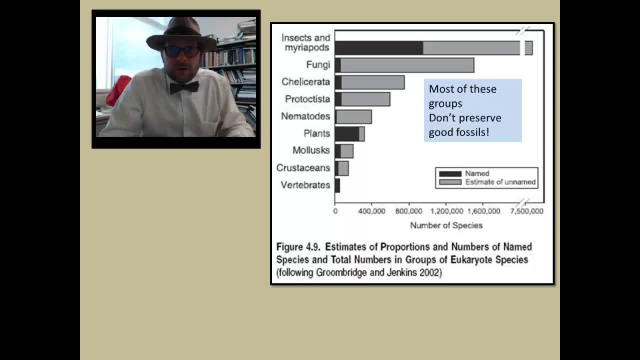 Paleontologists are quick to acknowledge that the fossil record of these groups are not spectacular and would never be able to reveal the true species richness in the fossil record. So rather than look at all the groups, let's narrow down to the 9 major groups that are: 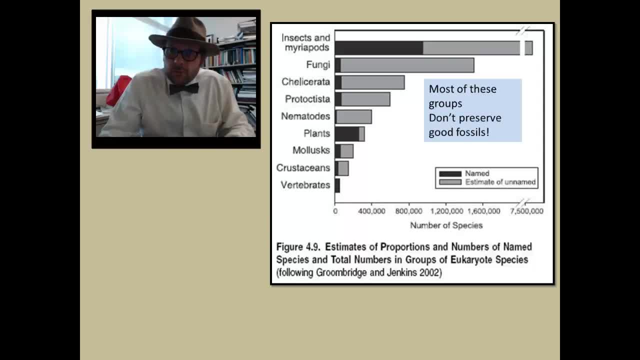 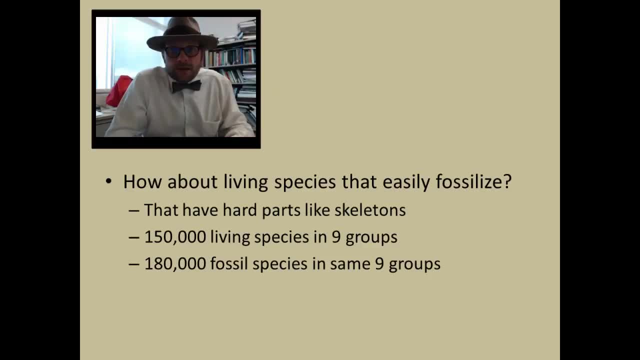 well represented in the fossil record: Life forms that produce hard parts, skeletons. they are easily fossilized. If we look at these 9 groups of life forms, we see that the numbers make a little bit more sense. The number of living species is 150,000, with fossil species higher and 180,000 species. 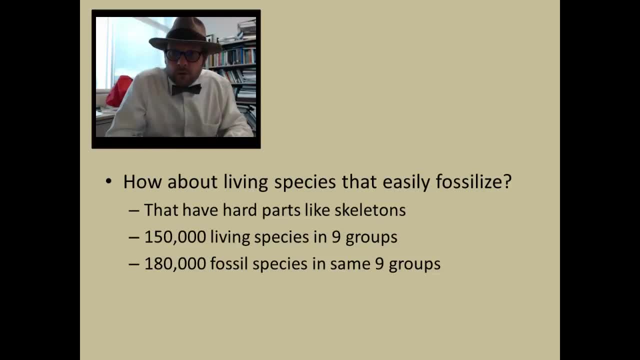 This means that the fossil record has a much higher proportion of the total number of known species. We can use the same calculations as before, using just these 9 groups, and we see that the fossil record is better. We can use the same calculations as before, using just these 9 groups, and we see that the fossil record is better. 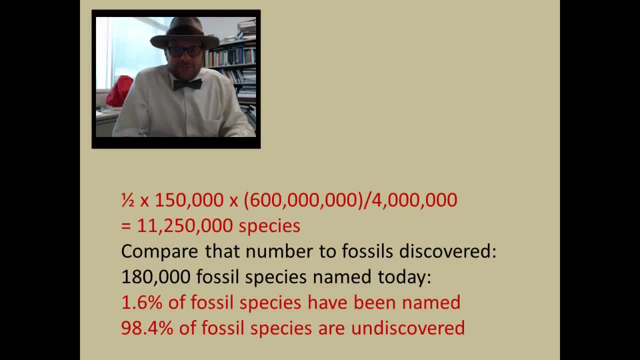 We can use the same calculations as before, using just these 9 groups, and we see that the fossil record is better: 1.6% of fossil species have been named and 98.4% of fossil species have yet to be discovered. 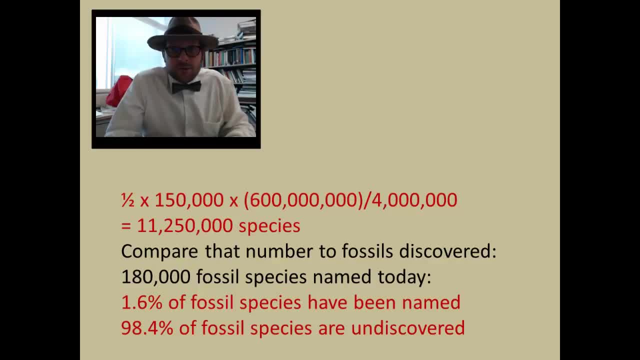 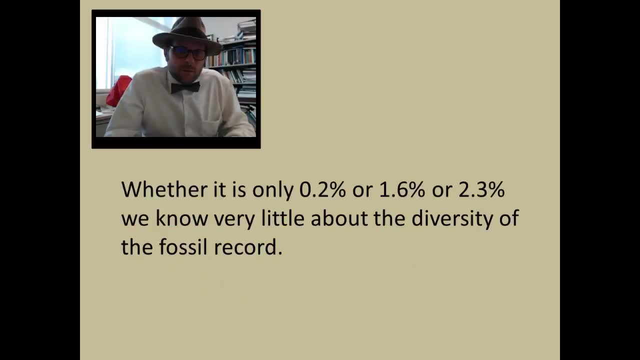 We still have a lot to discover in paleontology, if it is true, but these numbers are better than 0.2%. Whether it's only 0.2% or 1.6% or 2.3%, we know that these numbers are much better. 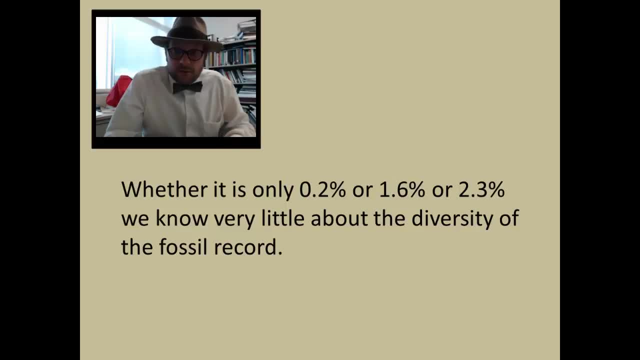 We know very little about the diversity of the fossil record. This is the biggest criticism of paleontology. This is why paleontology is rarely taught in science and it is rarely a requirement for a degree in biology. Paleontology is often viewed by the other sciences as having to deal with the fact that 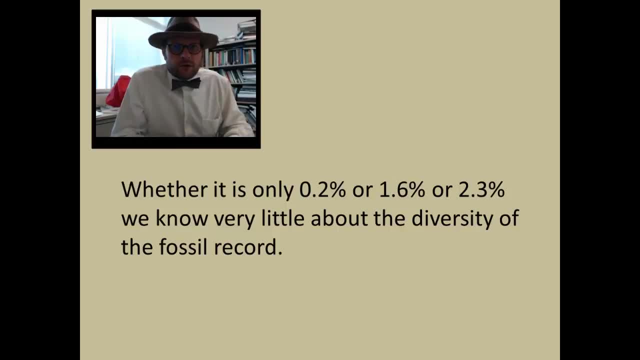 fossilization is extremely rare and that little can be discerned from the fragmentary fossil remains that are discovered. More so now in the age of molecular biology, molecular analysis and massive, huge data sets. the rarity of fossils and the paucity of fossil record seem to make paleontology 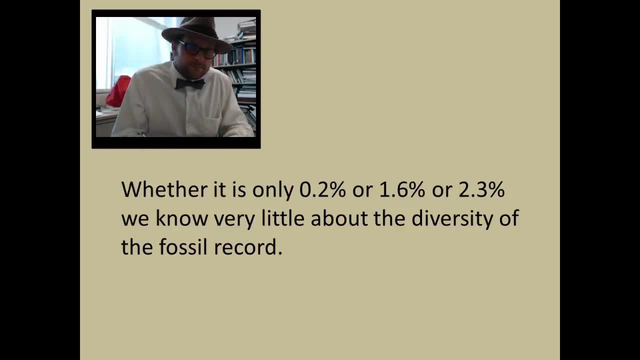 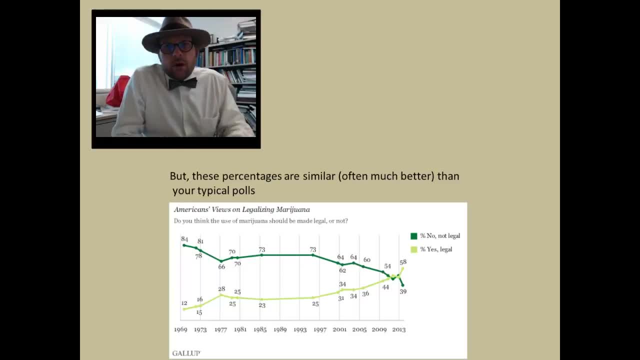 Question 3!. Question 3! Think about the value of polling data, where only a small percentage, often less than 0.2%- of a population is asked a question. for example, do you think the use of marijuana should be made legal or not? 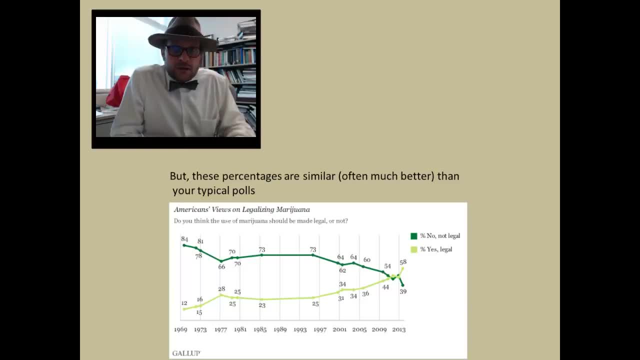 Of those surveys. trends can reflect the trends of the entire population, even if every single person was not asked that question. Hence, in paleontology, sampling and understanding the error associated with the sampling of fossils is critical to draw up the best conclusions from the available data. 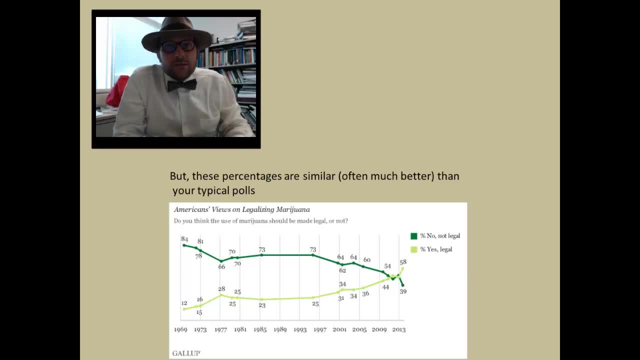 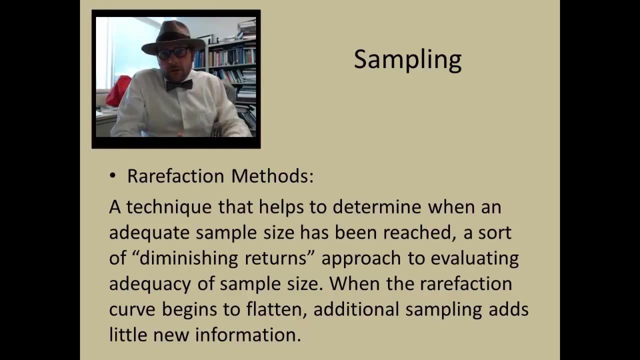 Paleontology is still critical to address questions that are not easily addressed by only studying living species. Let us look at one of the common ways to understand sampling in the fossil record: the rarefaction technique. Rarefaction technique helps to determine when an adequate sample size has been reached. 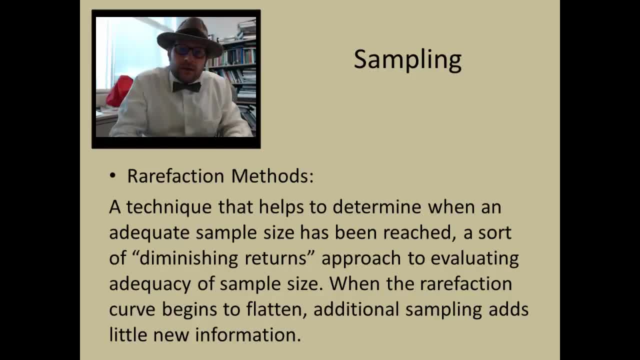 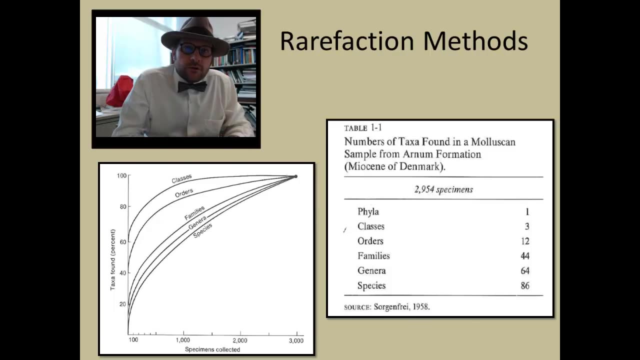 a sort of diminishing- Diminishing returns approach to evaluating the adequacy of a sample size. When rarefaction curves begin to flatten, additional sampling adds very little new information. The graph below shows the number of phyla reflected in rising numbers of fossil specimens sampled from the rock record. 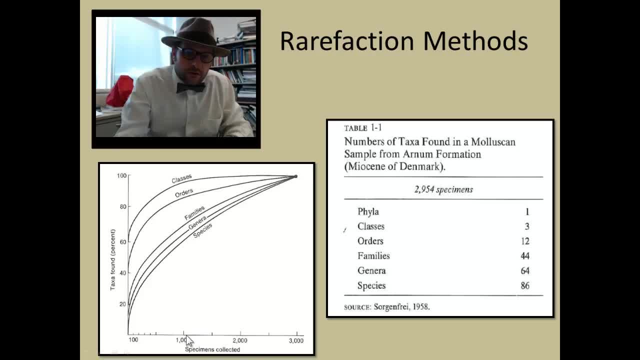 Note that as the number of specimens increase, which is the x-axis here, the number of species found increases. The total number of taxa found increases. But as you get more and more specimens, these curves begin to flatten such that if you collect 100 more specimens, the likelihood of discovering a new species decreases. the 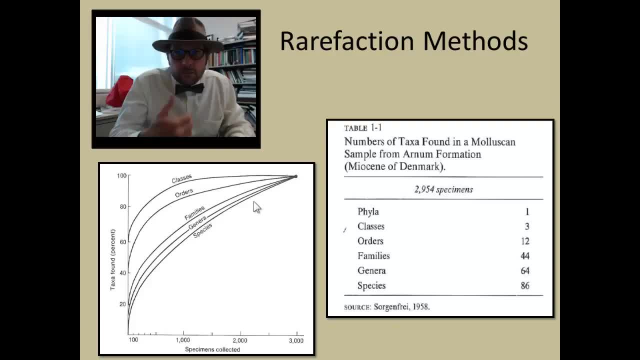 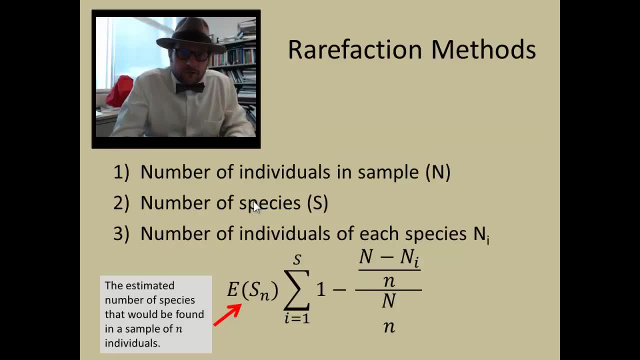 larger the sample size. Rarefaction is a simple formula to establish the number of species that would be found in a sample of n individuals. Rarefaction is a simple formula to establish the number of species that would be found in a sample of n individuals. 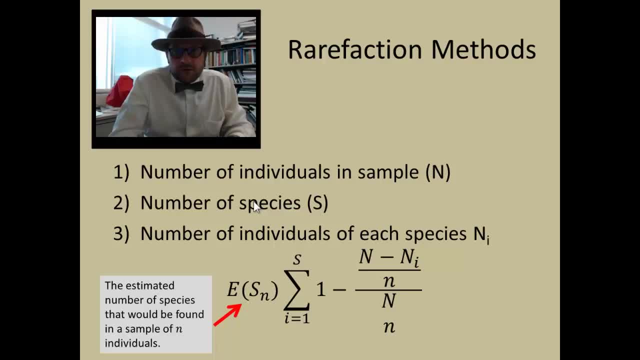 The number of species is n, the number of species is s and the number of individuals of each species is ni. This summation equation will give a good estimate of the number of species. Let's look at an example of using this equation. 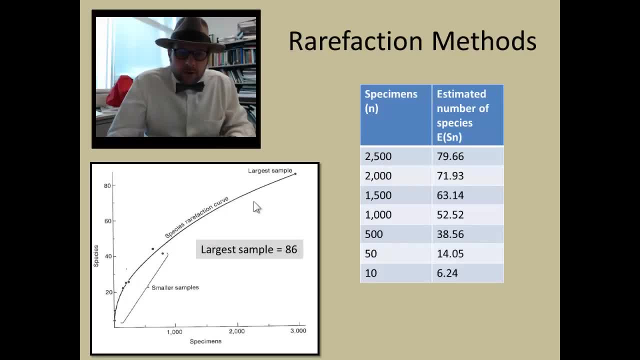 In this example we have a number of sets of data where we have gone out and collected a bunch of fossil specimens. From that collection of specimens we then figure out what species are found in the sample size. We then separate them out into separate species. 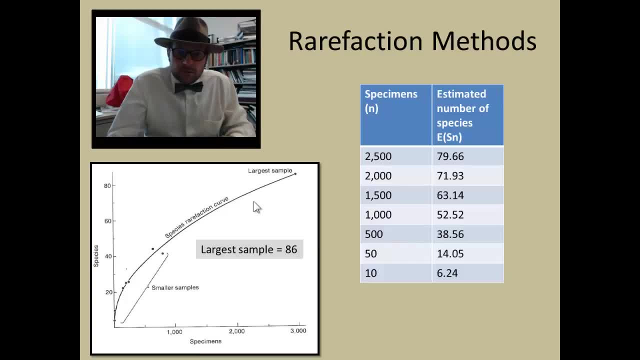 We will talk a little bit more about what a species is and how to get about doing this. What you will notice is that the sample size- that is, the largest sample, which is close to 3,000 specimens here- has the largest number of species- 86.. 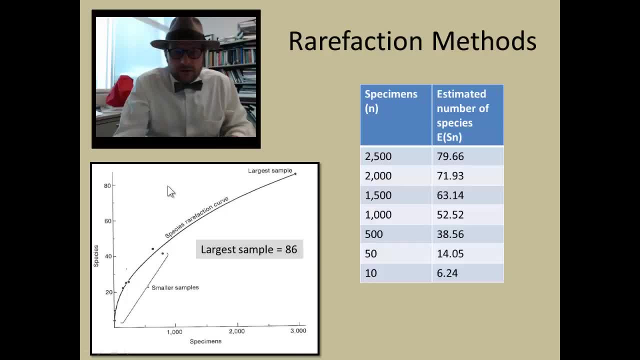 Of the 3,000 fossil specimens that were collected, 86 were unique species. The number of species is 86.. The number of species is 86.. The number of species is 86.. One of the things we can do is, if we have a number of these samples, we can calculate. 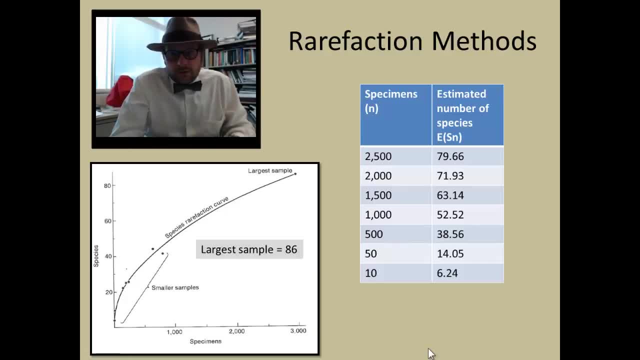 the estimated number of species using each one of these sample sizes. This way we can put error bars, or what we can do is figure out how many specimens we have to collect before we can be satisfied with the number of species that we have actually captured in our sample. 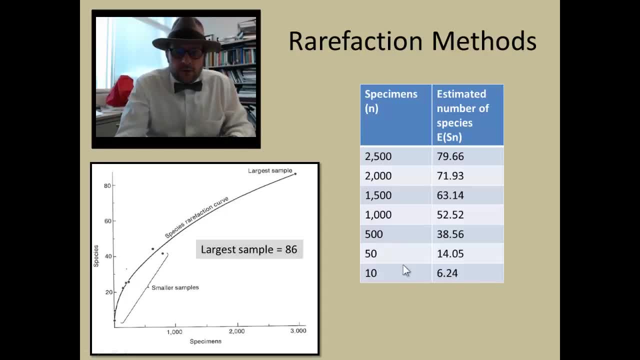 You will note that in this chart, if we look at the number of specimens, we can see that of specimens, as the number of specimens increase, we start to get closer and closer to that 86 number. So that's when we're going to get things start to level out and flatten in the curve. 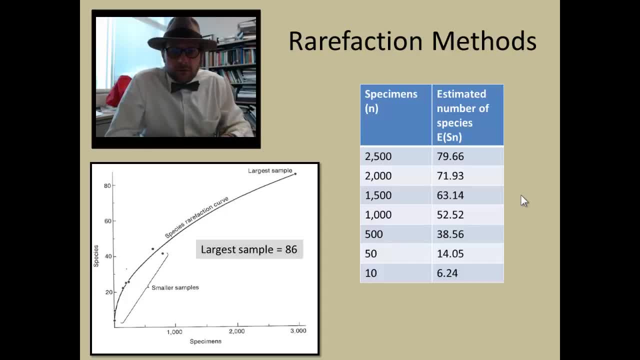 So you can use these curves. To do this in practice is sometimes difficult. Often times you have to do this on the best sampled locality or horizon and then use that to basically see how other sites compare to that site that you're looking at. But ratification is a really powerful tool and it's very useful in determining how well sampled you are. 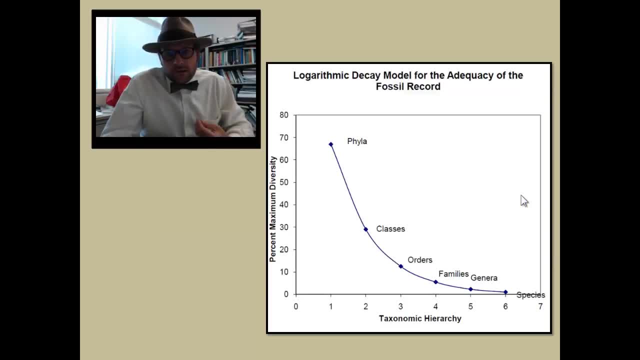 Now one of the interesting things that can happen is that if you look at different hierarchical groups- so if you're looking at whether you have representatives of different classes or orders, or families or genera, you'll note that you'll note that you'll note that as your sample sizes increase, 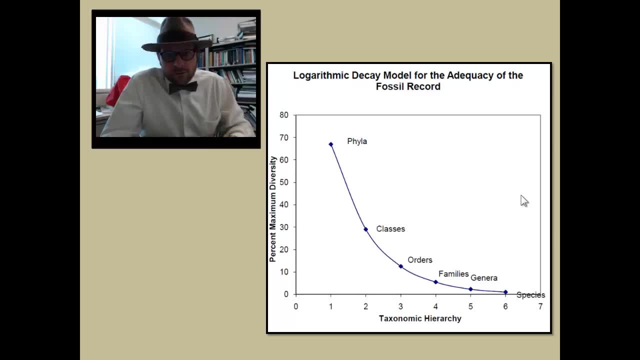 you're more likely to capture all the classes than you are all the species, And this is just because of this logarithmic, decay model. looking at different groupings, Now, often this transcribes itself into studies that look at families in genera, rather than species. when you're looking at diversity through time studies, 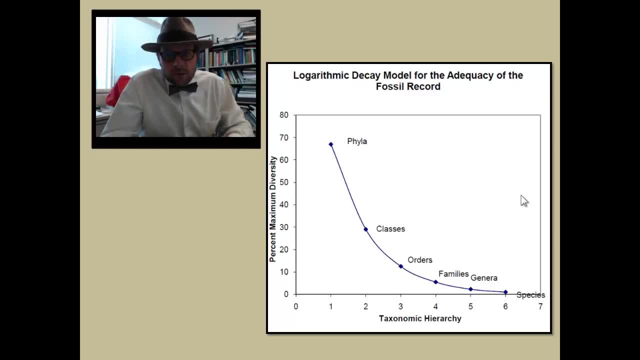 So, for example, this Dabansky curve used the marine invertebrate record to look at diversity through time rather than species, because the fact that you're going to capture all the species in the fossil record is less likely than capturing all the families in the fossil record. 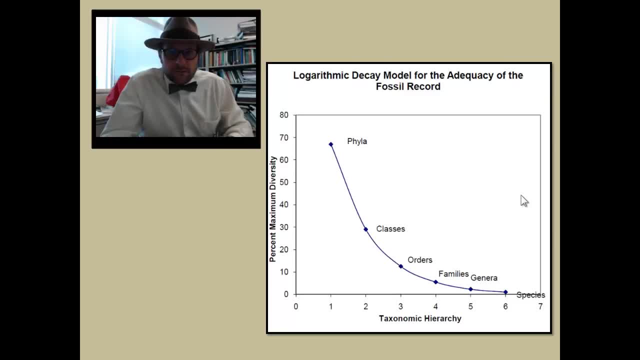 So there's this decay model of preservation that you see. So often times paleontologists will use genera or families or orders, even and less likely species, although that's starting to change More and more, paleontologists are starting to be able to get pretty good species numbers. 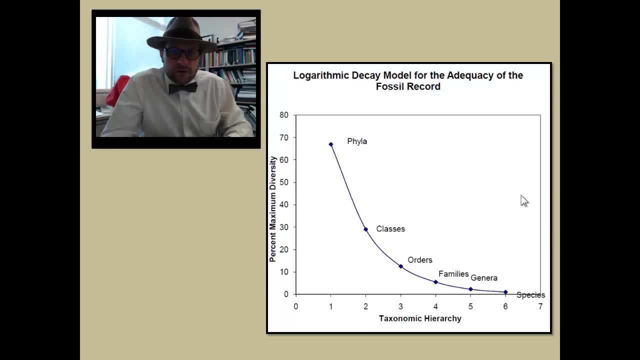 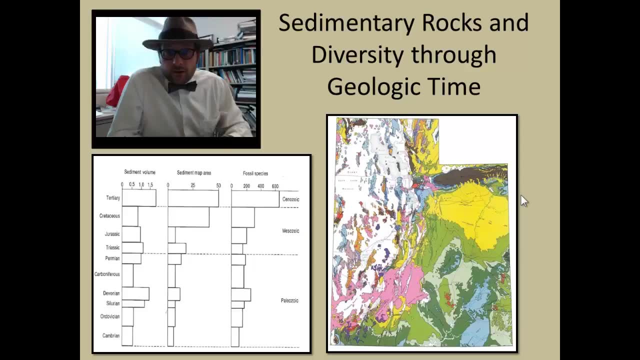 based on these larger sample sizes that are being generated Now. this is not the only way to take a look at how good the fossil record is. Another way to look at how good the fossil record is is by looking at the geographic exposure of rocks at different time periods and comparing that with a fossil record. 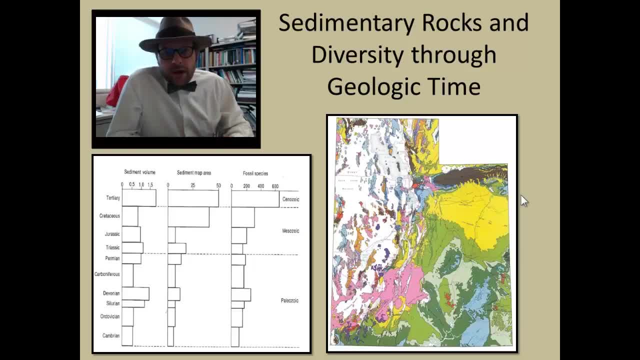 So one of the things that's been observed is that the farther back in time you go, the more likely it is that you're going to get a fossil record. So one of the things that's been observed is that the farther back in time you go, 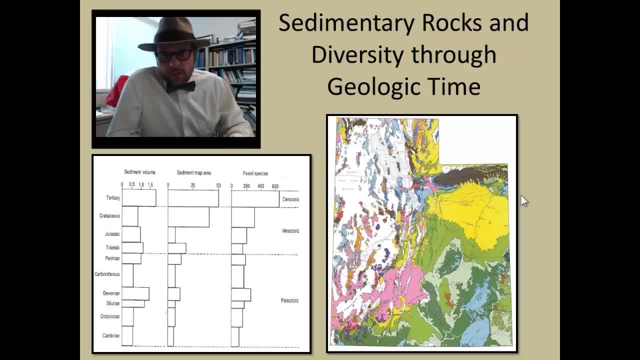 the less exposures of the rock of that appropriate age is. So, for example, if you're interested in studying the Cambrian here in Utah, there's a few places that you can go along the Wasatch Front where you can find some great Cambrian fossils. 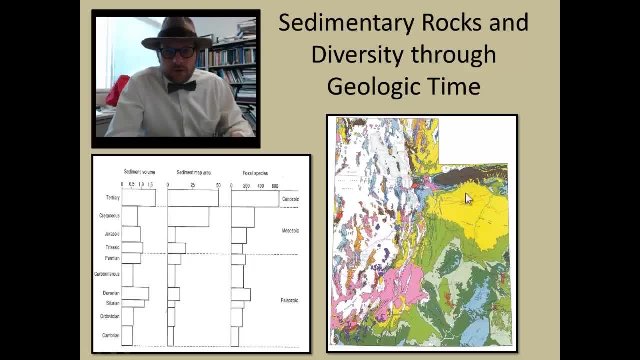 You can find them out in western Utah and a few places along the Uinta Mountains. But if you're interested in studying a much more recent period of time, say the Cenozoic or Cretaceous, for example- the Cenozoic is the yellow rocks here which you can see occupies a huge portion of the state. 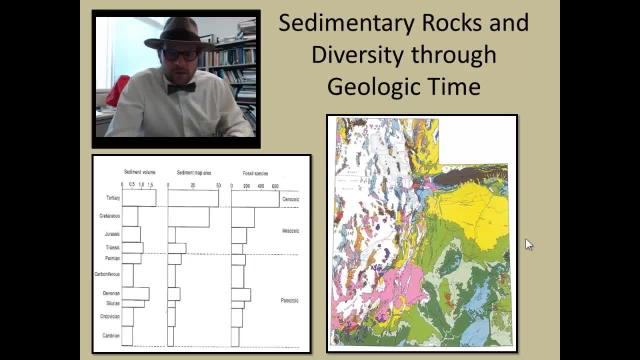 The green indicate the Cretaceous and Jurassic rocks, which are also fairly well exposed compared to the Cambrian. So one of the things that people begin to do with these geological maps is sort of quantify the amount of sediment that's out there of each one of these to try to use that to play around with how good the fossil record is. So one of the things that people begin to do with these geological maps is sort of quantify the amount of sediment that's out there of each one of these to try to use that to play around with how good the fossil record is. So one of the things that people begin to do with these geological maps is sort of quantify the amount of sediment that's out there of each one of these to try to use that to play around with how good the fossil record is. 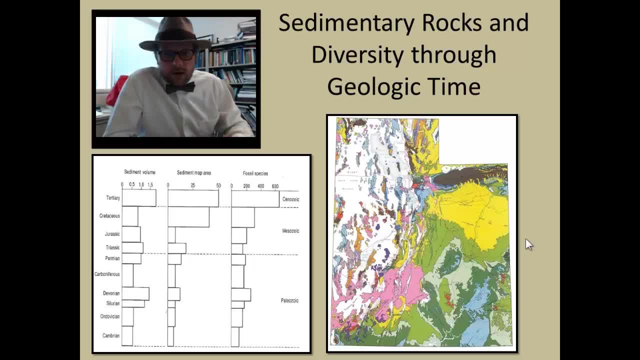 So obviously the fossil record of the Cenozoic, those yellow rocks, are much better than Cambrian, which is the dark purple rocks that we see, So more exposures that we can look at. So this is another way of estimating how good the fossil record is. 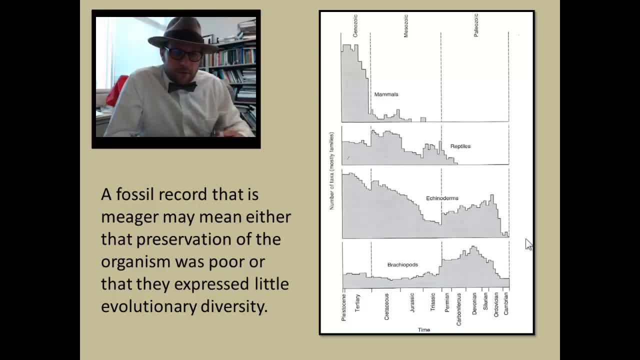 Now, a fossil record that is meager may mean either that preservation of the organisms is very poor or that they express little evolutionary diversity themselves, And this has been a huge debate within paleontology, For example. here we're looking at the number of taxa, so this is mostly at the family level through time, of various groups. 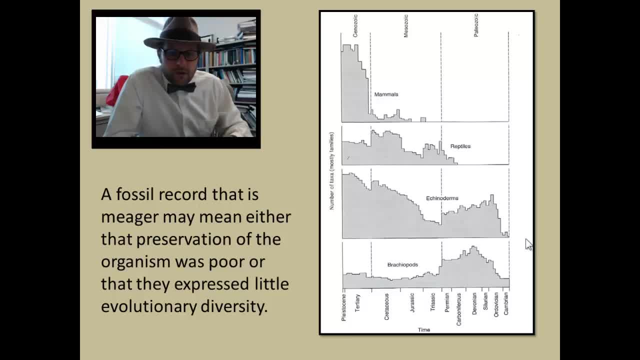 We've got mammals, reptiles, echinoderms and brachiopods. One of the things you kind of notice is that, for example with mammals, that after the extinction of the dinosaurs at the end of the Mesozoic era, 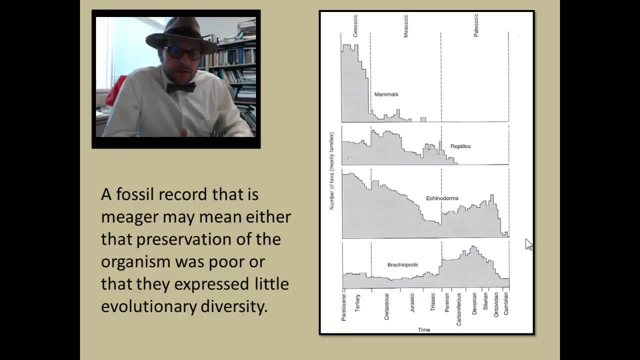 we have the proliferation of mammals in the Cenozoic. Some scientists have debated that, in fact, this big jump in mammal diversity at the end of the Mesozoic is just an artifact of poor sampling and that, in fact, many more mammals in the Mesozoic have yet to be discovered. 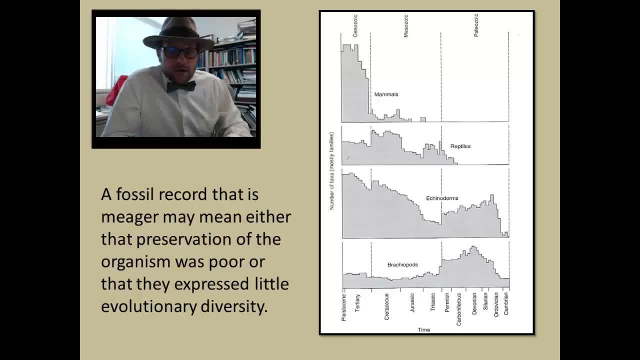 And the reason that we don't see them until after the Cenozoic has to do with preservation. The same could be true with brachiopods. You see a huge proliferation of brachiopods in the earlier period of time and maybe the fact that we don't see brachiopods in the Mesozoic- they're less diverse. 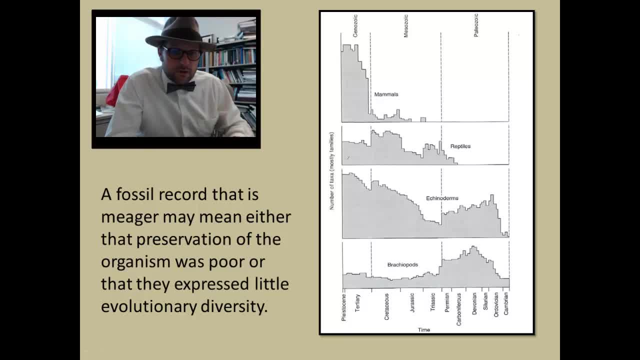 may have to do less with a change in the population. The change occurred at the Permian-Triassic boundary and may have something to do with the fact that brachiopods are just not well preserved in the Mesozoic, for whatever reason. 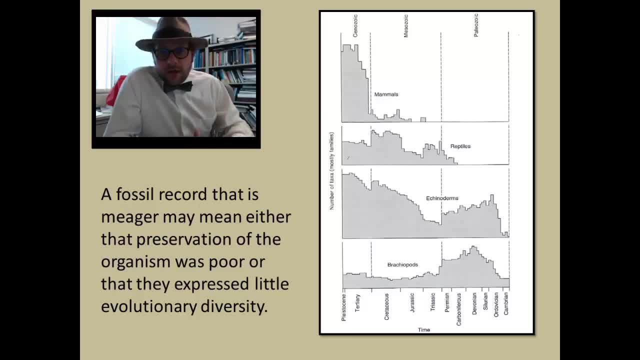 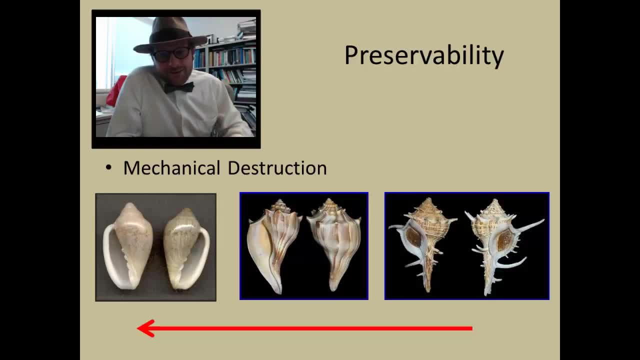 Paleontologists that view that the fossil record is pretty good at reflecting the data will argue that this is just a reflection of the actual evolution of the species of spines coming off it, a very ornate shell If it's tumbled in a surf or broken up on a beach. 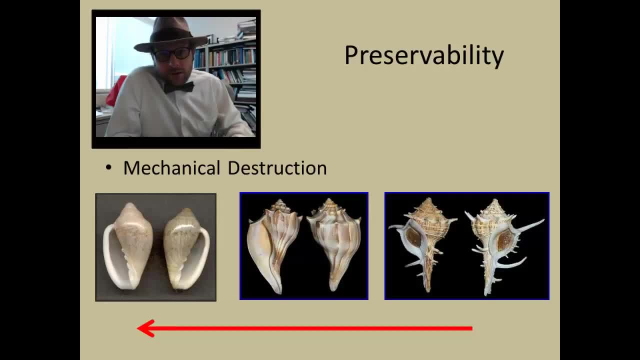 those pieces are going to easily break off of it and it may not preserve very well. Yet if you have a shell that doesn't have any of that ornamentation, really thick and robust shell, then it will likely survive a lot of that metallical destruction and it will be. 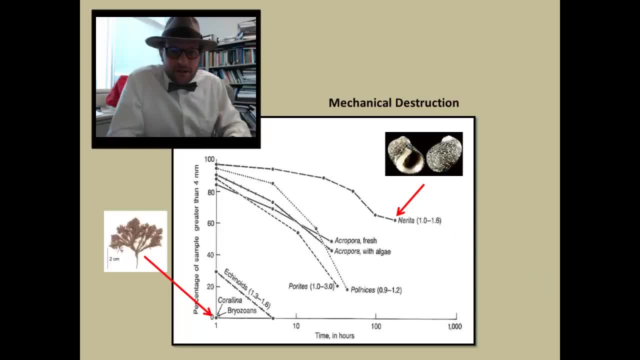 better represented in the fossil record. There have been some really fun experiments looking at mechanical destruction. Here's an example, one that's in the reading. For example, here the scientists took a number of different organisms that they found living along a nearshore marine system. It included this gastropod Netrita. 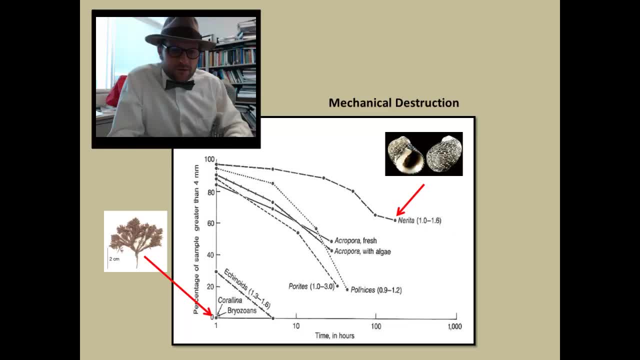 that they threw in, but it also included bryozoans and corellia, which are the ones that they found living along a nearshore marine system. It included this gastropod, Netrita, that they threw in, but it also included bryozoans and corellia, which 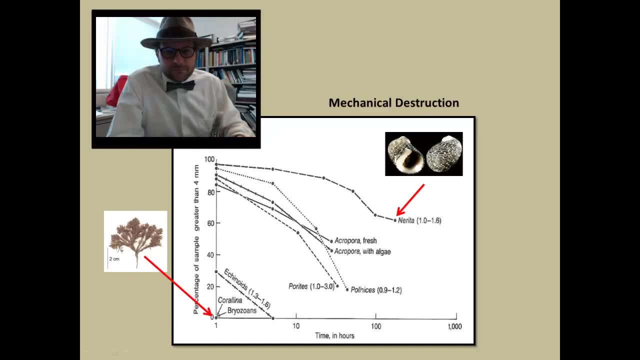 is this very fan-like, very brittle coral. They threw it in there, tumbled it and within just a few minutes that was blown apart. They did it over time and then calculated how much of the sample was represented by each of these groups. What's really interesting is that the Nerita survived clear out here over 100 hours. 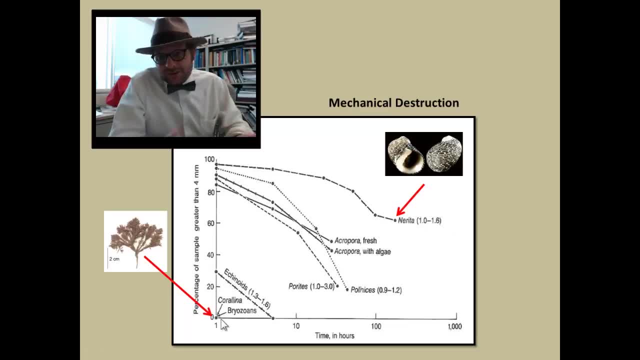 whereas these bryozoans, these more brittle organisms, just didn't make it into the fossil record. So if this is representing the fossil record, you're often sampling, not sampling the more brittle types of fossils that just don't get preserved in the fossil record, The ones that have 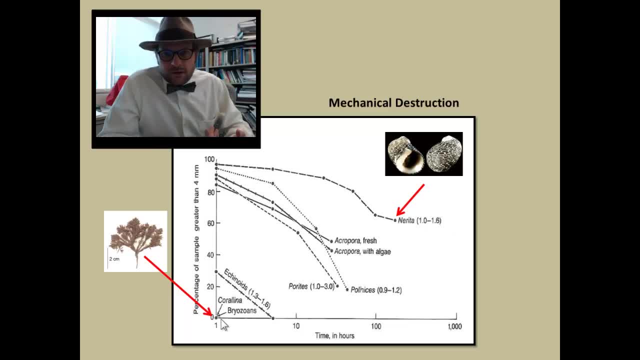 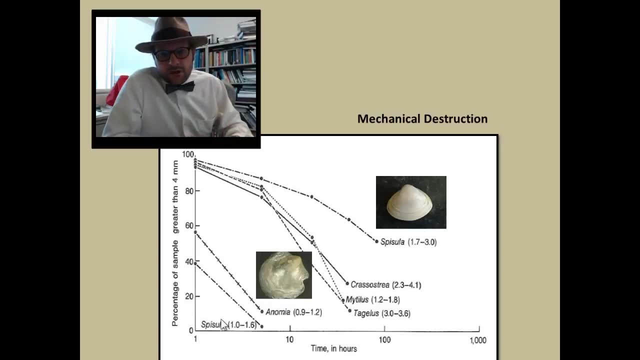 robust, strong shells are going to be the ones you're going to be over sampling. Here's another example, in this case not necessarily looking at differences in the shells, but also kind of how the shells are constructed as a whole in Maine are made, and you can see that over time as they tumble these in a rock tumbler. 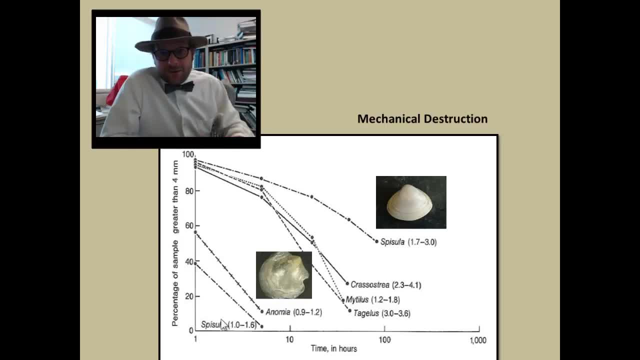 some of the clams are able to survive, whereas the oysters tend to get busted apart into teeny little pieces and weren't as well represented, and eventually get disintegrated when the rock tumbler keeps tumbling and tumbling and destroying these things. 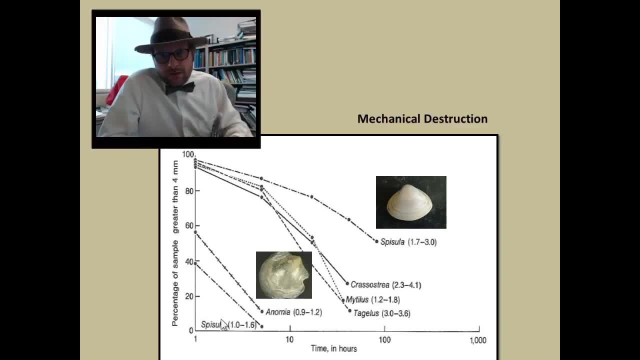 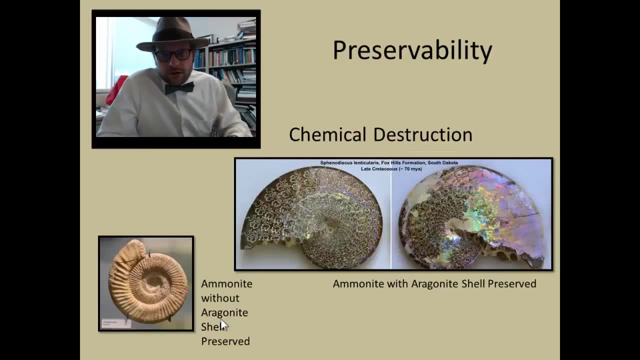 So some wonderful experiments have been done to looking at the taphonomy, that is, the sampling of each of these things, And these are things to be aware of when talking about the fossil record, Talk about chemical destruction. So one of the things that we'll discuss throughout this class is that various organisms compose. 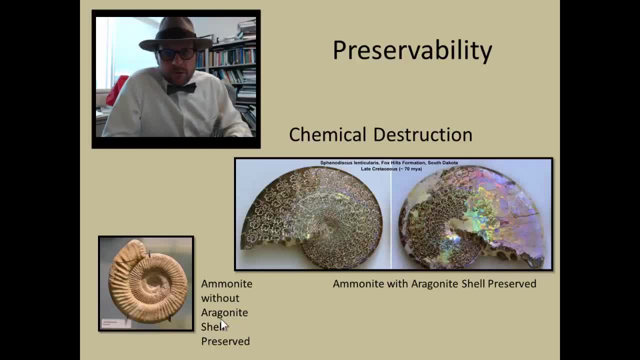 their skeletons of different types of minerals. Most of them do with aragonite, but other organisms produce skeletons of silica or calcite. Aragonite doesn't like to sample. They stick around when it's in the subsurface. It's a very delicate crystal lattice structure that's used in aragonite. 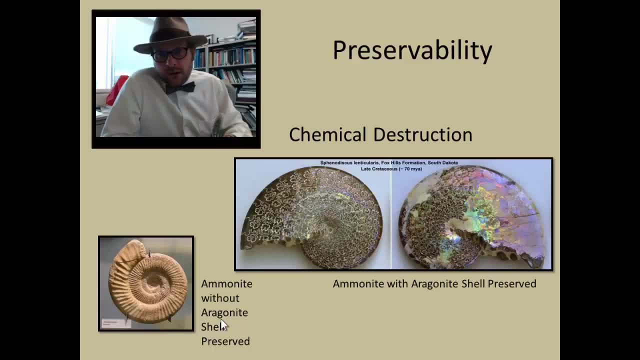 And so when these fossils get buried, they tend to recrystallize into calcite or get completely dissolved. So in this example, here we have an ammonite with the original aragonite shell preserved, and that gives it that really cool, shiny sort of mother-of-pearl effect. 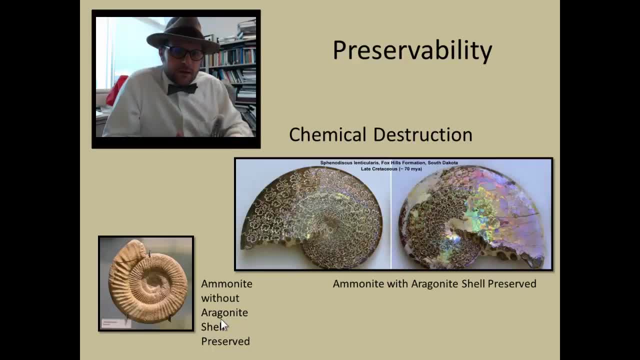 And then here below we have the very dull ammonite without the aragonite shell. In fact they probably had a very pretty mother-of-pearl sort of look with the aragonite on the outside of that ammonite shell, but it's just dissolved away, quickly dissolves away in groundwater. 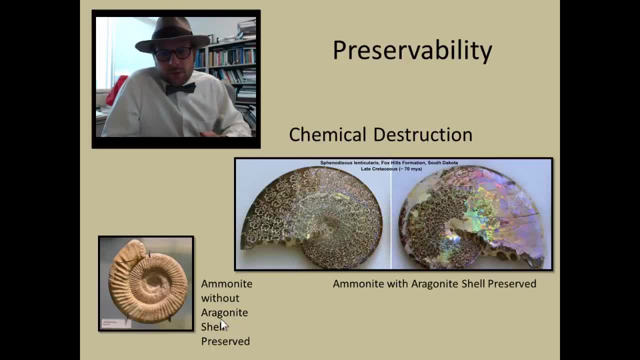 even if it's just a little warm, The groundwater will totally replace or take away that skeleton. So chemical destruction is very common in the fossil record, oftentimes altering the skeleton as it's being preserved. So one of the things that PAMELAcom is doing-